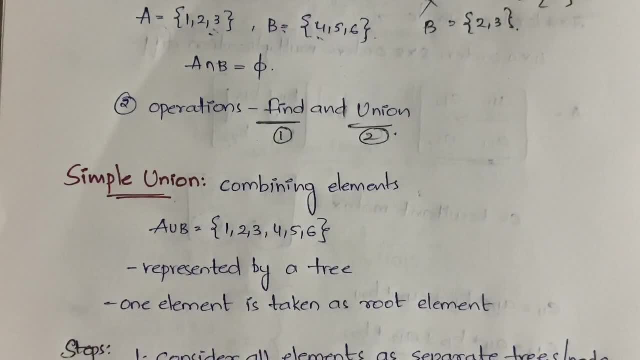 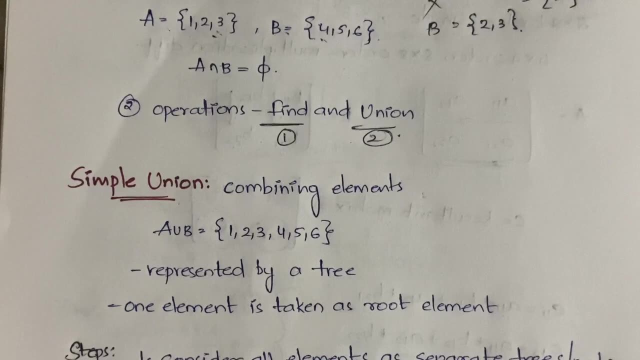 3,, 4,, 5, 6.. Union means simply, you are combining all the elements. Repeated elements you will take only once, But since we do not have any repeated elements here, you can take all those elements as such. Okay, we are representing this union operation with the help of a tree, Okay, and 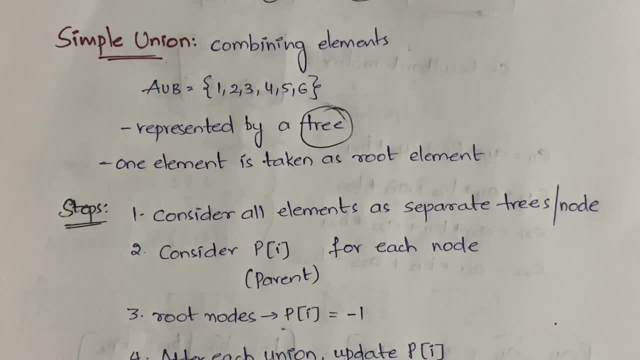 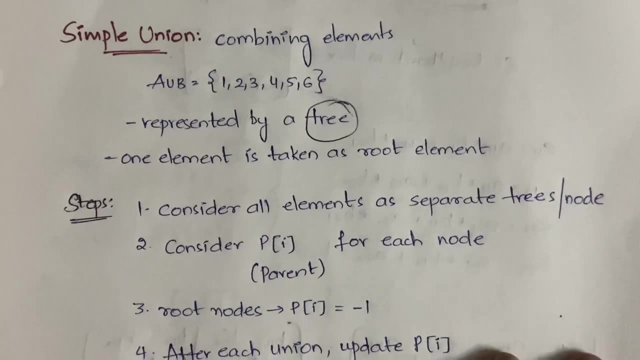 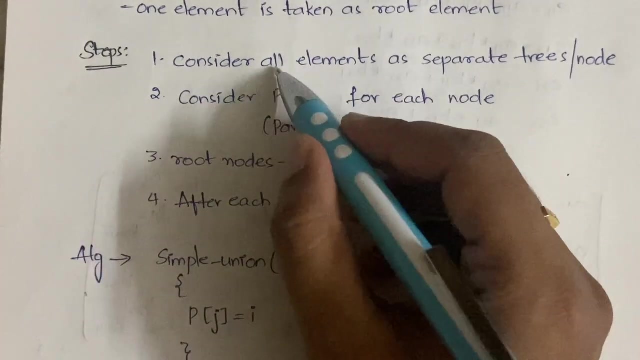 among all the elements. you can pick any one of the element at the root node Arbitrarily. you can pick any one of the root element as the root node Done. So now let us see what are the steps we have for the union algorithm. First, you have to consider all the elements as separate trees or 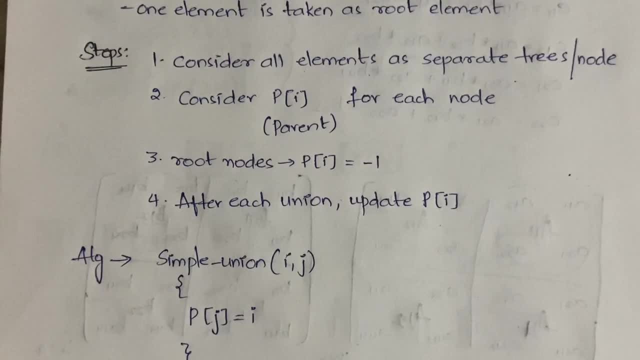 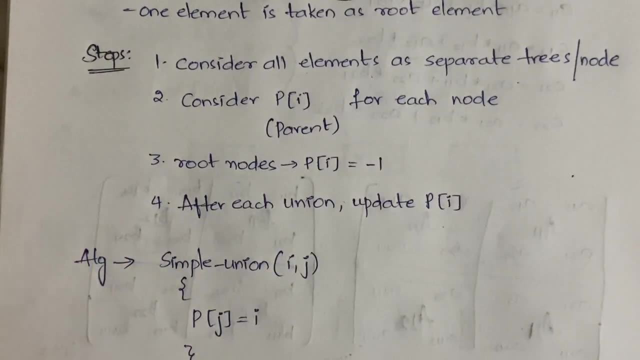 separate nodes. You have to consider each and every element as a different node. Okay, then you have to consider P of I for each node. How you will consider P of I, I will tell you: P of I is nothing but what. 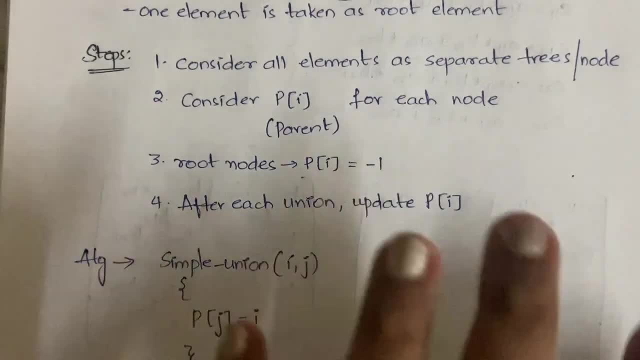 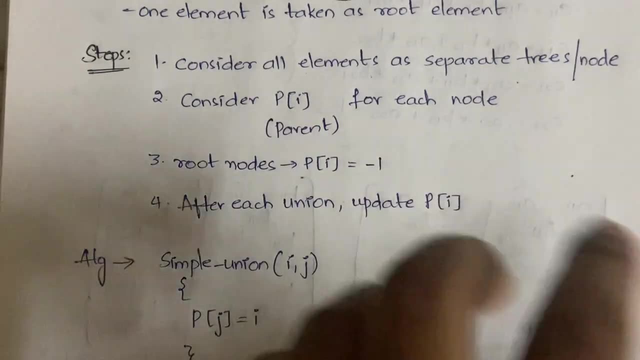 Parent value: Okay, the parent value of each and every node you have to consider. Next, for all the root nodes, you have to initialize with the value of minus 1.. Okay, minus 1 should be initialized to all the root nodes And after each and every union operation. 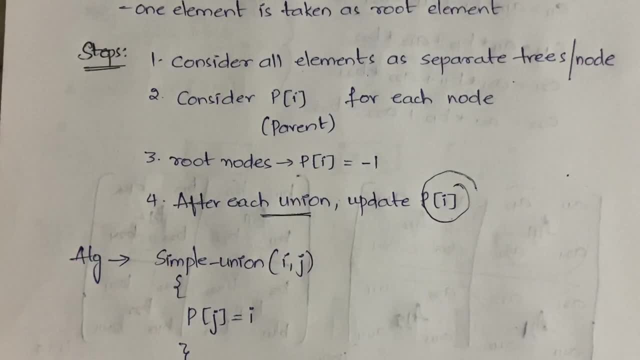 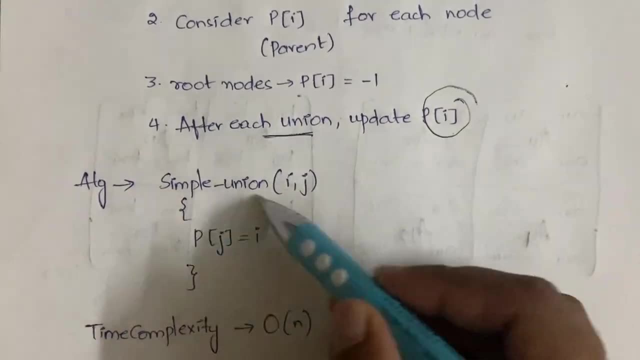 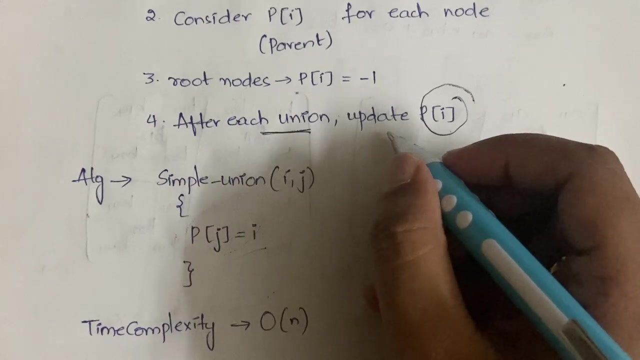 you have to update your P of I value. How you will update your P of I value also, I will tell you with example. Don't worry, This is the algorithm, simple algorithm, Just one step. P of J is equal to. don't worry, I will tell you how to do that. Okay, so what he said? first he asked you to 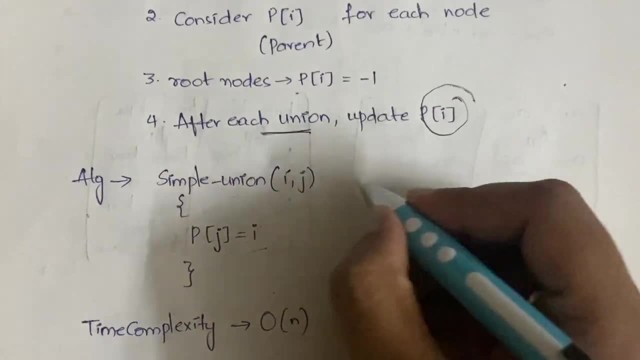 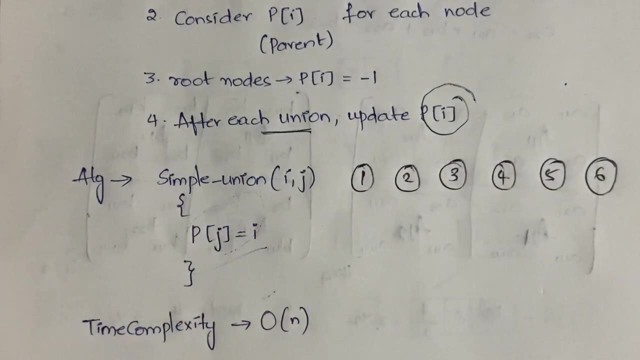 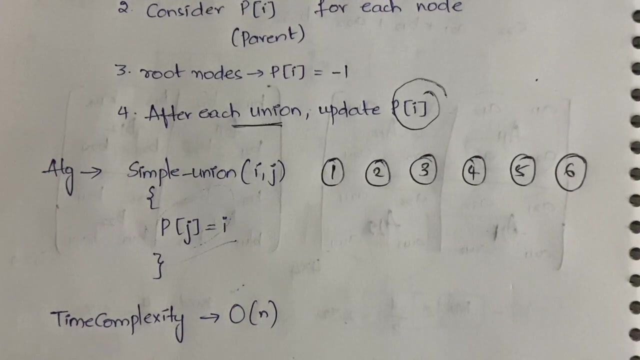 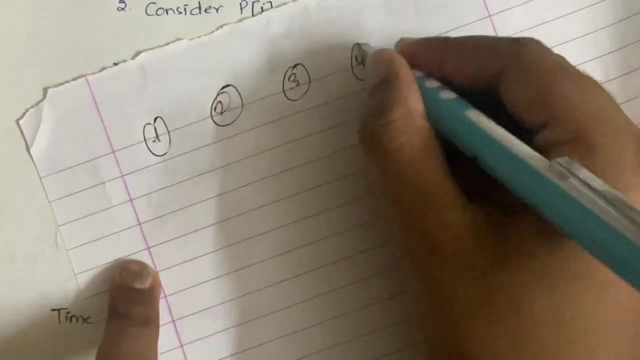 assume all the elements as separate nodes, right? So let us take 1,, 2,, 3,, 4,, 5 and 6.. Okay, now what you will do is: let me take another piece of paper. Okay, now what you will do: 1,, 2,, 3,, 4,, 5, 6.. 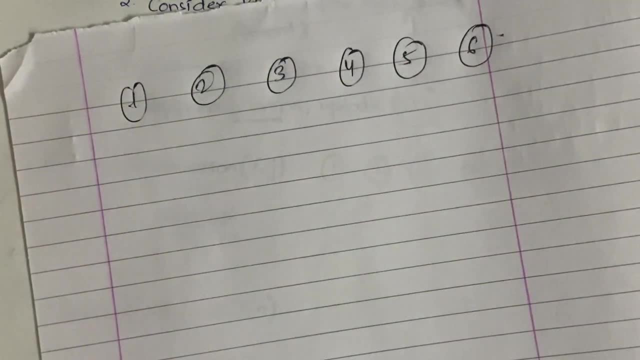 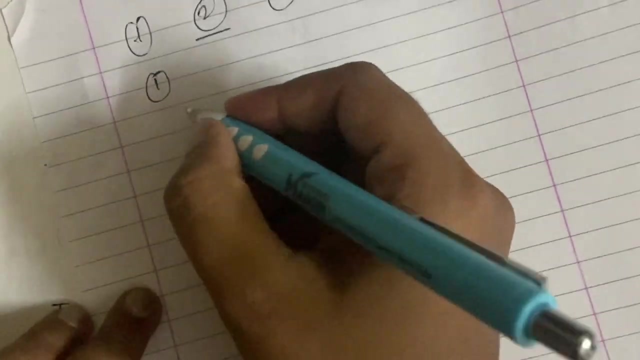 So each and every element, you have assumed it as a different, different nodes. Okay, now you will be combining two, two elements. Two, two elements means what? First, you will take 1. And you will combine 2 with 1.. That means like this: Next, you will take 3.. You will combine 4.. 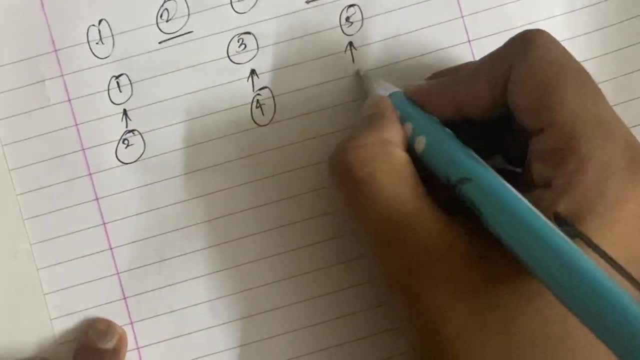 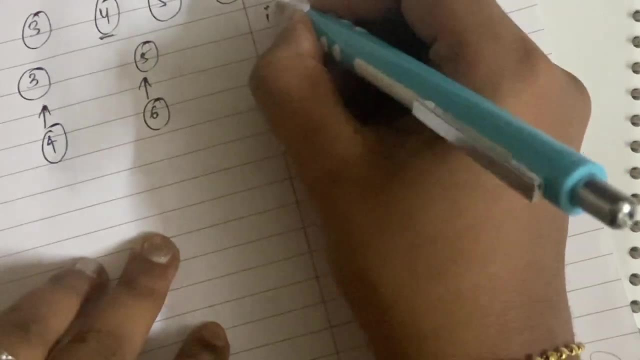 Okay, next you will take 5.. You will combine 6.. Okay, in the first step you did this. Now we will have this is I value? Okay, this is 1,, 2,, 3,, 4,, 5, 6.. 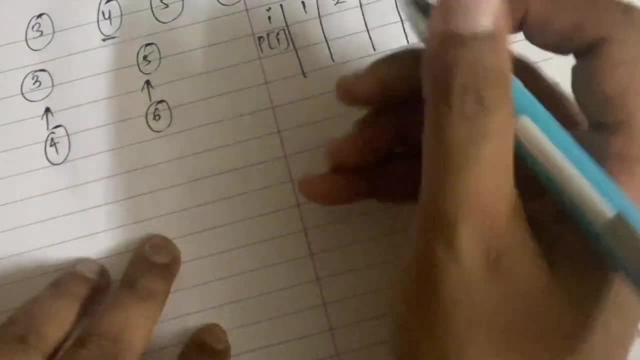 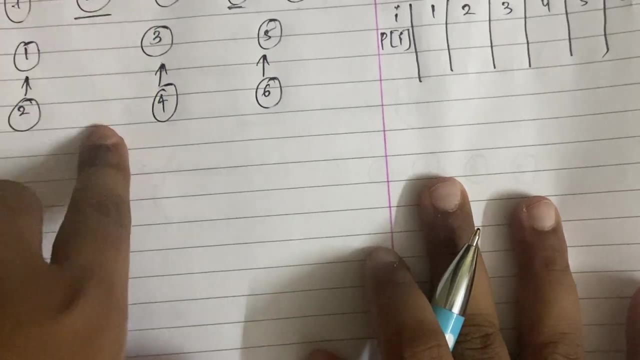 Now what is the P of I For the first iteration? Okay, so who is the parent of 1? There is no parent. 1 itself is the parent node right. So for parent node or root node, what we are taking P of I value as: 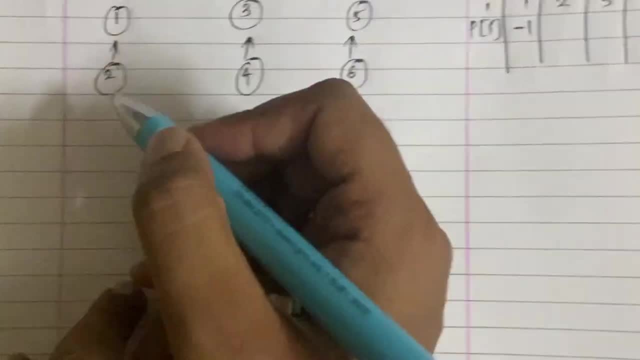 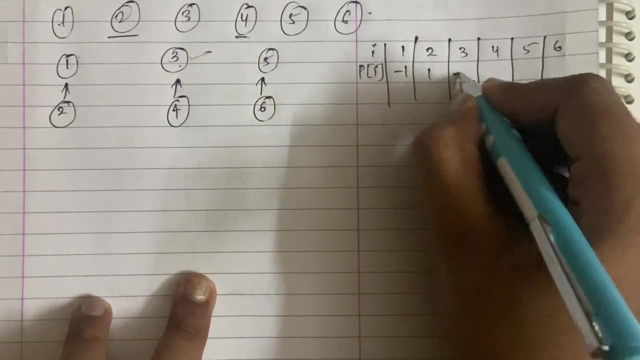 minus 1.. So here you will have minus 1.. The parent of 2 is 1.. Okay, next Parent of 3, P3 itself is a root node, So minus 1.. Parent of 4 is 3.. 5 is a root node, So minus 1.. 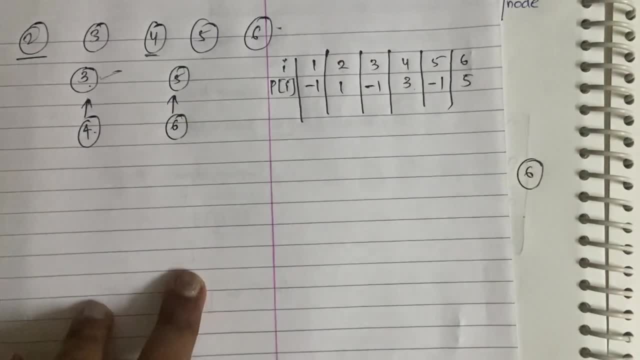 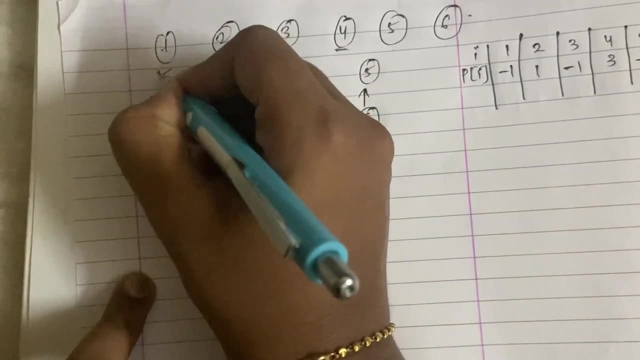 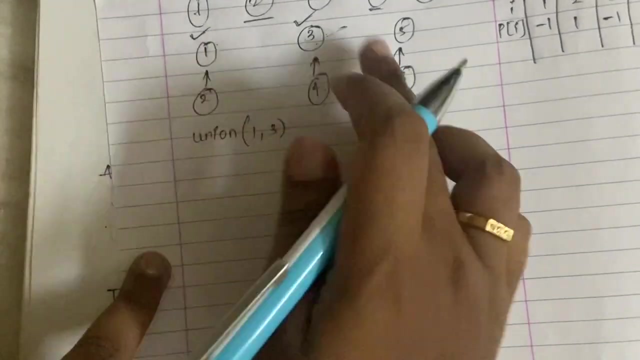 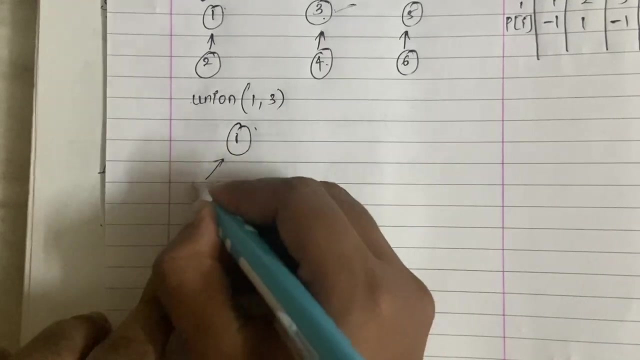 The 6. Parent is 5.. Okay, done So. this is the first iteration. In the second iteration, what you are doing, You are combining this tree and this tree. That means union of 1, 3. We are taking only root nodes. Okay, that means what you will do now: 1, 2.. Now what you are. 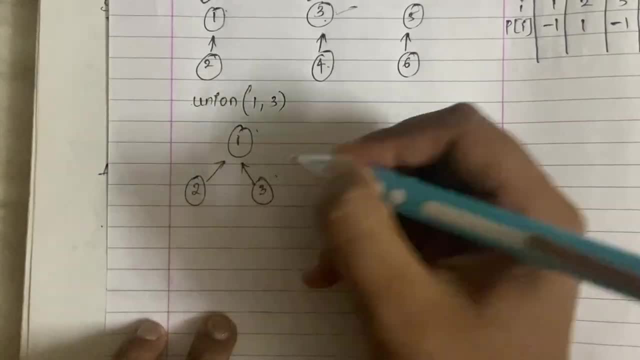 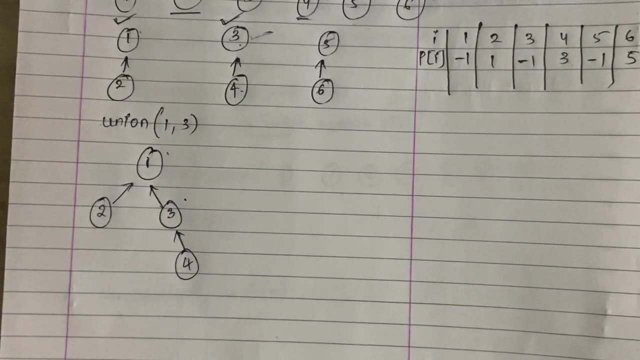 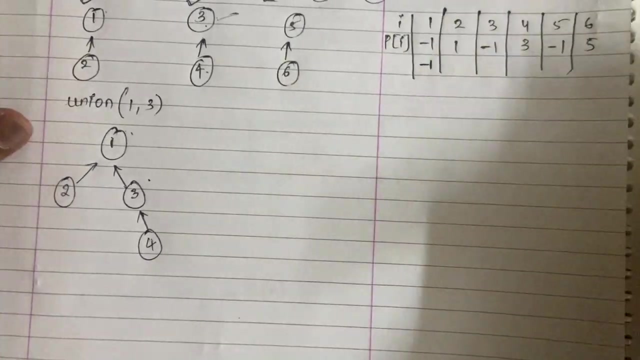 doing. You are joining 3 here. Okay, just simply. you are joining 3.. And for 3, you have 4.. Okay, So now again, update the values here. I is the root, sorry, 1 is the root node, So minus 1 as it is Next. 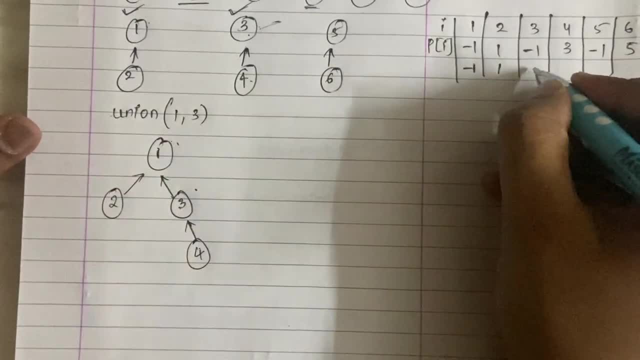 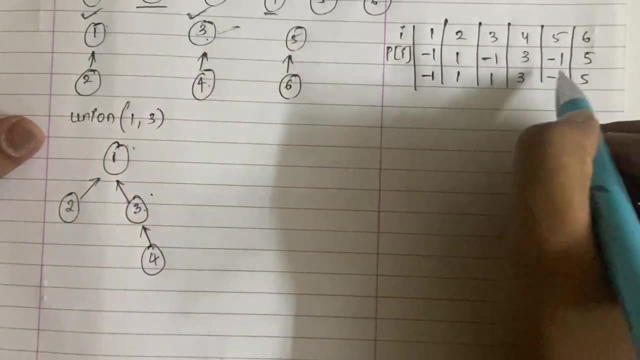 Who is the parent of 2? 1. Parent of 3? 1. Parent of 4? 3. And 5 and 6, as it is Okay, because 5 is the root node and 6, the parent of 6 is 5.. 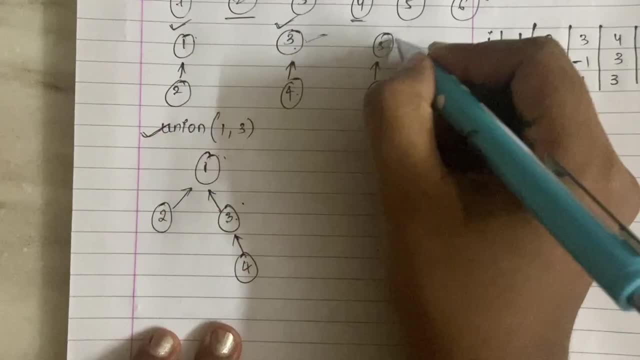 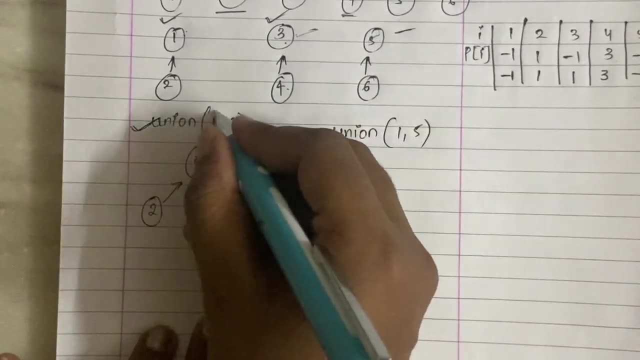 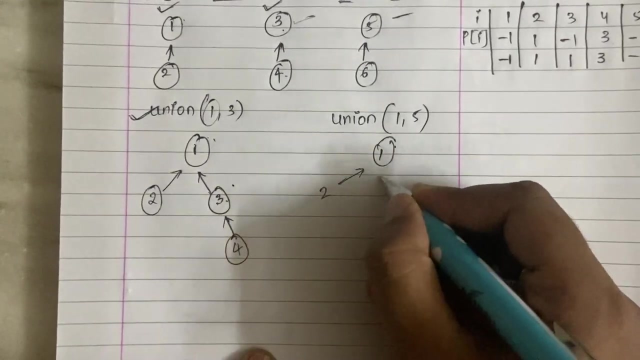 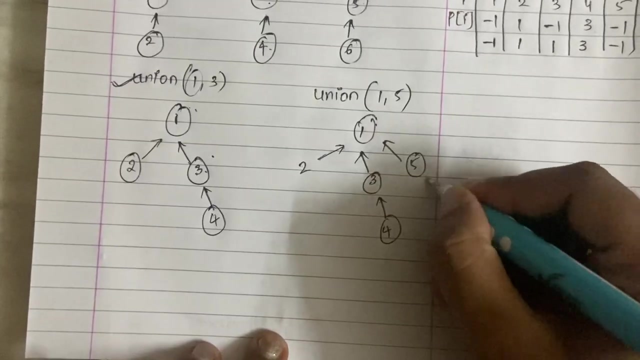 Now what you are doing. You are combining this tree and this tree. Okay, that means union of 1, 5.. You are just representing the root nodes, Okay. So this tree, you will take it as it is. Next, here 5 will come, And then here 6 will come. So now see 1. 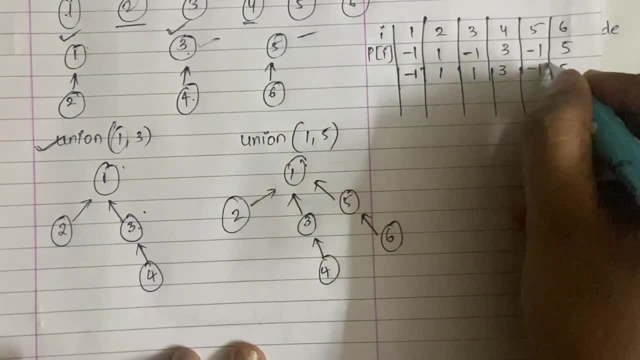 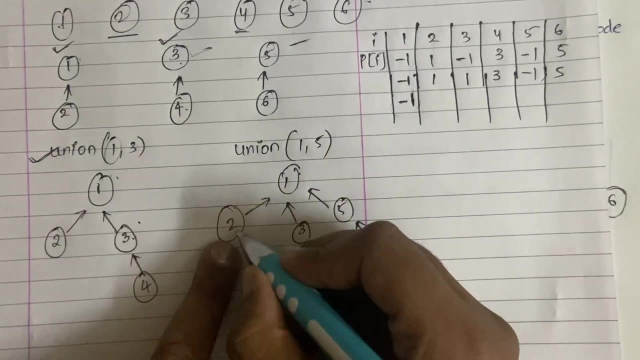 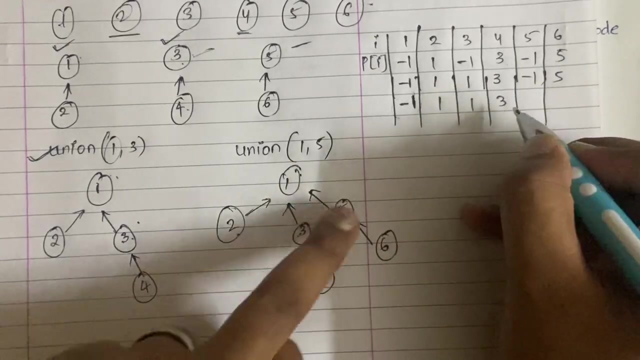 as it is is because one is the root node. ok, so minus one for root node. you should always give minus one, right. so minus one as it is next. who is parent of two? one who is parent of three? one, parent of four is three, parent of five is one and parent of six is five. ok, done so you. 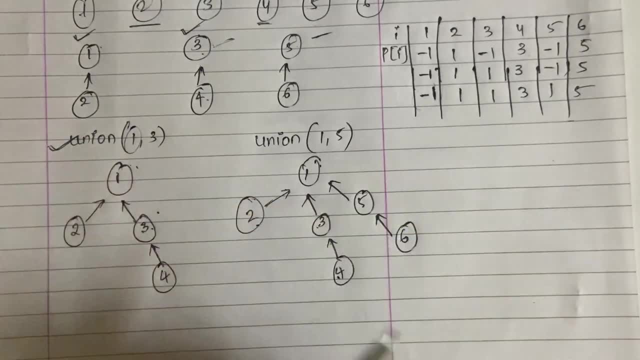 have covered all the nodes right, so union operation is done. this is how you will do union operation: very, very, very simple, ok. simple logic. you have to keep adding all the sorry, keep combining all the nodes until all the nodes are completed. this is simple union. that is why it is very simple, ok. next you will have weighted union also, but for now, let us. 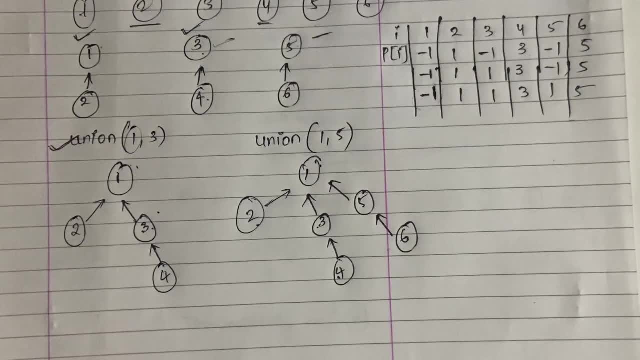 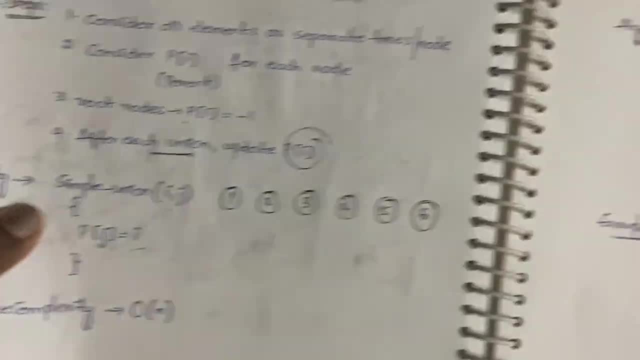 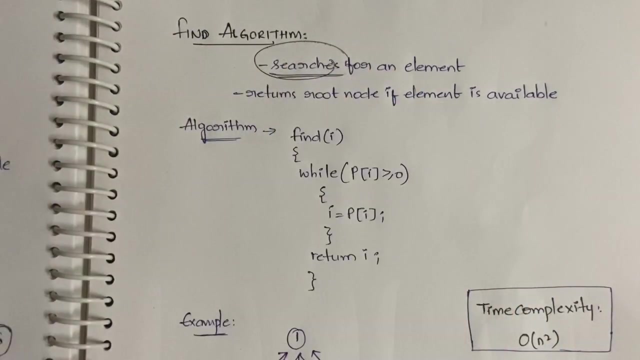 see find and the next videos. we will learn about simple, or i mean weighted union and collapsing find, and all ok. Now let us see the find algorithm. so find means what? basically you are searching for an element. ok, find means you are searching for an element like quick sort, merge, sort, what we did there. we are sorry. 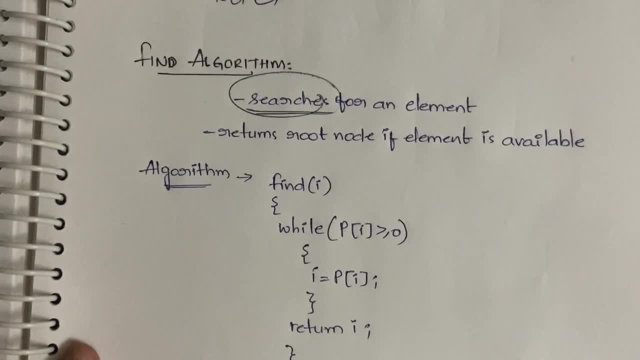 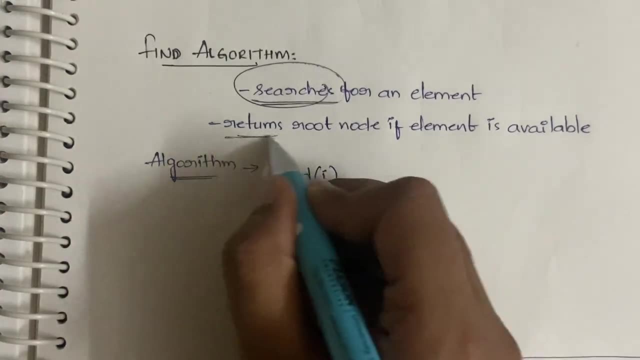 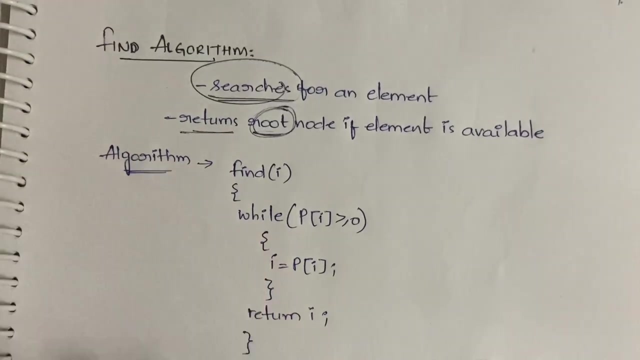 not sorting binary search, linear search. what we did? we just searched for an element. right here also, you are searching for the element only. so here, what you will keep getting, you will get the root node of the element, for example, in here, not here. where was our example? 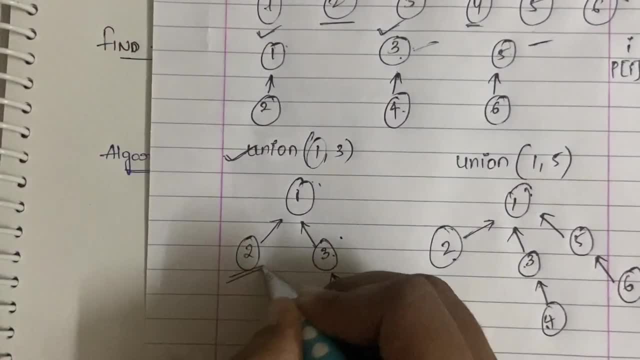 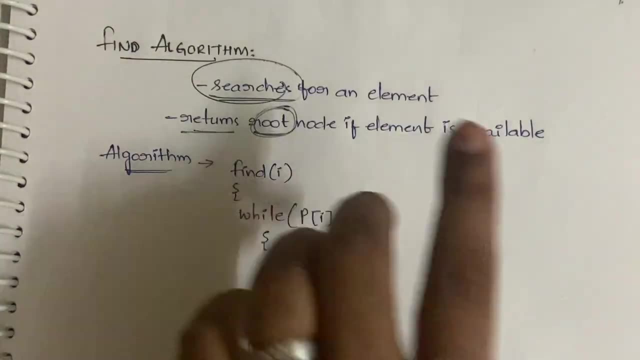 yeah, here, for example, you are searching for element two. then what it will return? it will return one. the root node of the respective element will be written if the element is available. if it is not available, we cannot do anything. ok, so the algorithm will be like this: find. 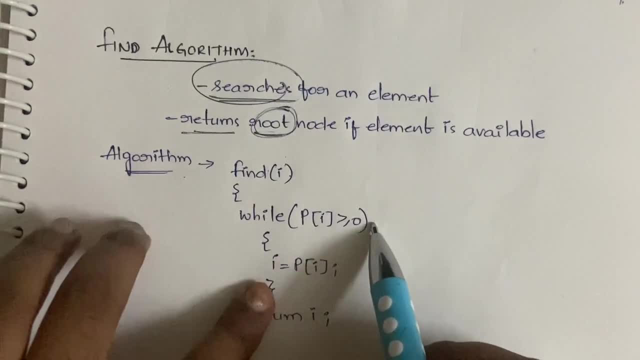 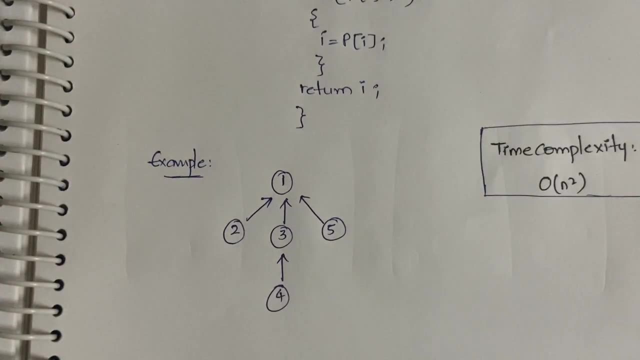 of i, like what you are trying to find. if p of i is greater than zero, guys leave this algorithm. i will explain you the example, then i will explain you the algorithm, then you will understand it clearly, otherwise now you will not understand it properly. ok, ok. 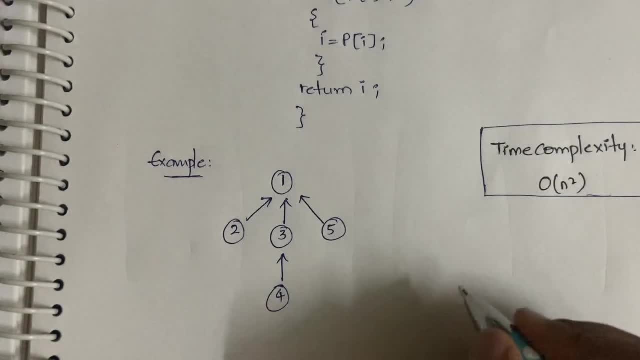 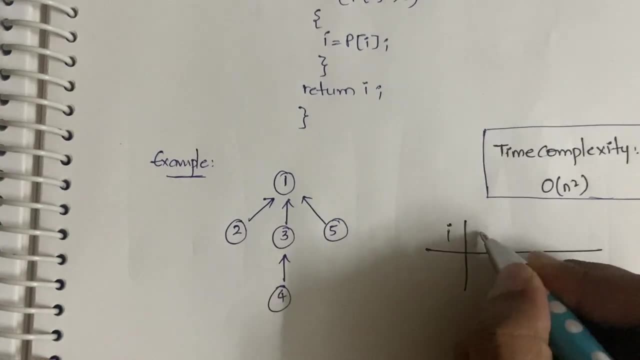 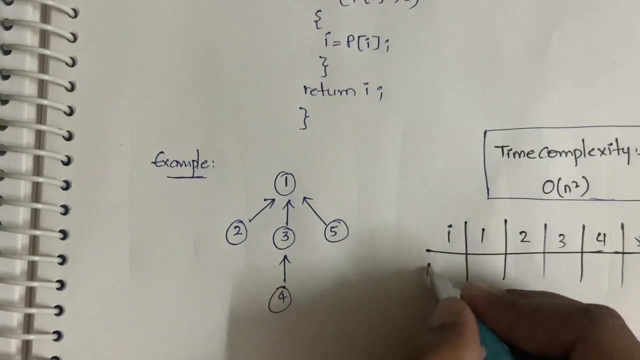 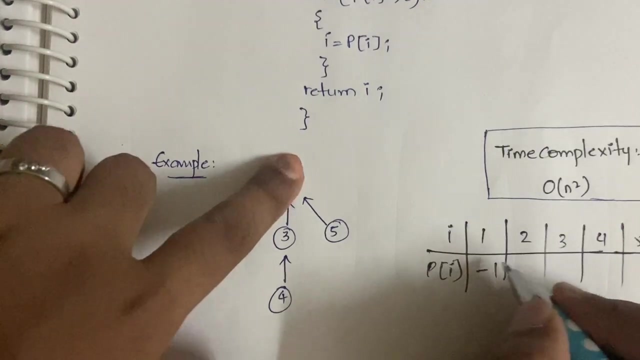 done. see first, just do the same. what did we do the matrix previously? one, two, three, four and five. ok, in p of i. so what is p of i? for one, it is minus one because it is the root node, and for two, the parent is one. for three, parent is one. for four, parent is three and. 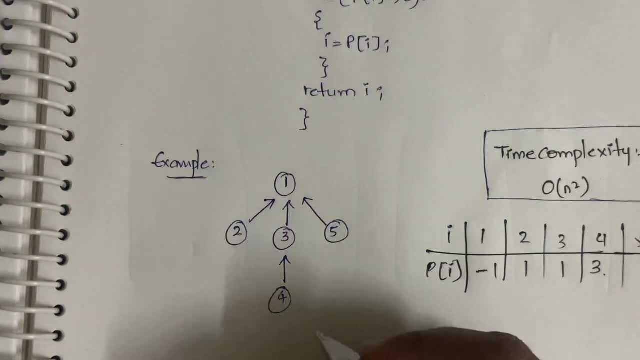 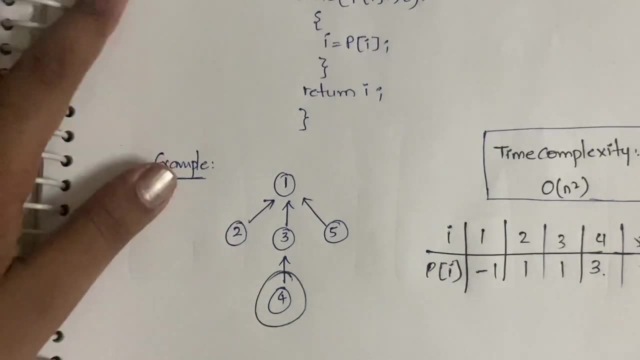 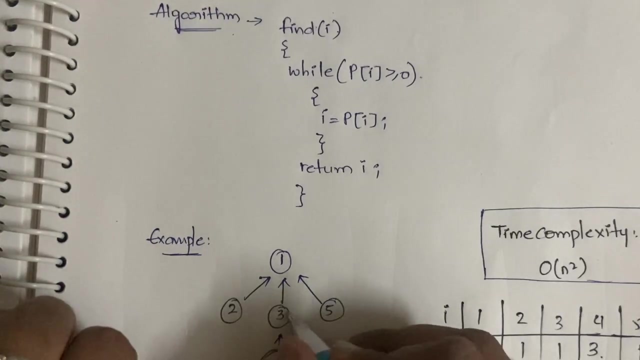 for five parent is one, ok, ok, For example, we are trying to find four, we are trying to find the element four, ok, so what we have to do? first, we have to find the value of the parent of four, who is a parent of four, three. so 3 is greater than, or equal to zero or not. yes, it is greater than of equal. 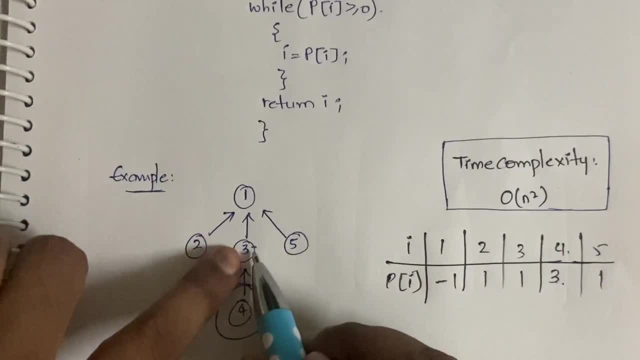 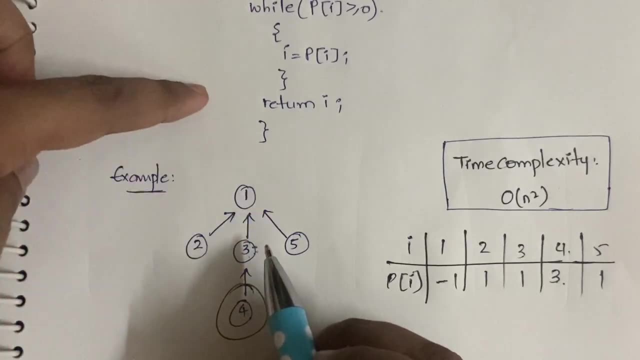 to zero. right, the parent of four is three. and now find out the parent of three. who is the parent of three? one One is greater than or equal to zero. yes, next, who is parent of one? the parent of one is minus one. minus one is greater than or equal to. 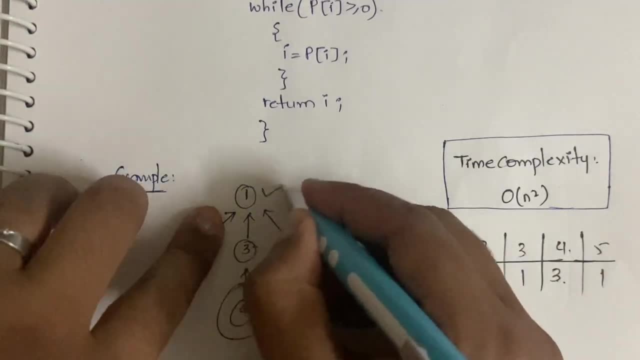 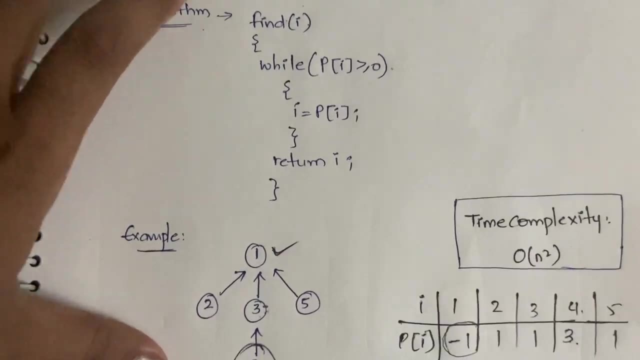 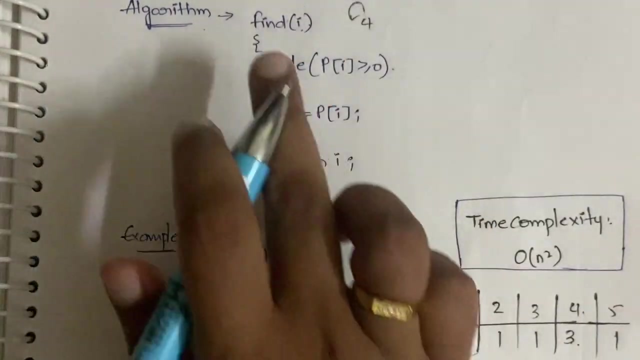 zero. no, it is not so. that means one is the root node. one is the root node for the element four. i will explain you with this algorithm now. suppose you are trying to find four, so you are passing four as the parameter. so find of four, while p of i is greater than or equal to zero, p of i means what? 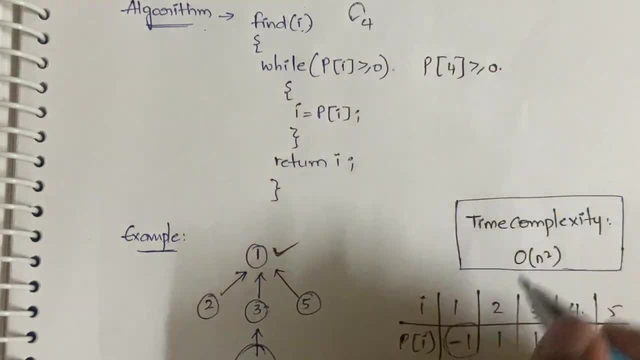 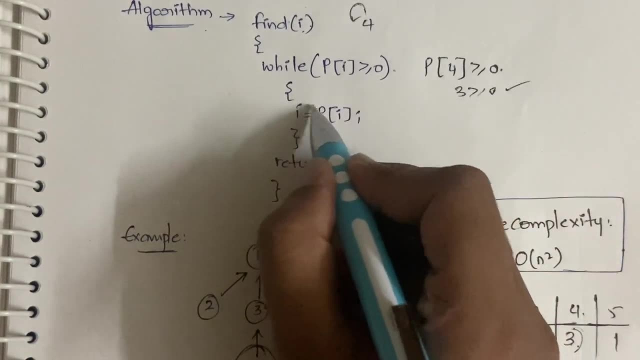 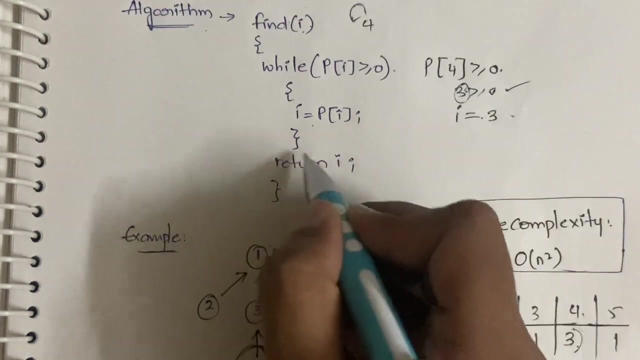 p of four is greater than or equal to zero. check: p of four is three. three is greater than or equal to zero. true, now what you have to do. i is equal to p of i. that means i is equal to how much? now p of i is what? three? so i is equal to three. again, go back here, here, so find of three, now your. 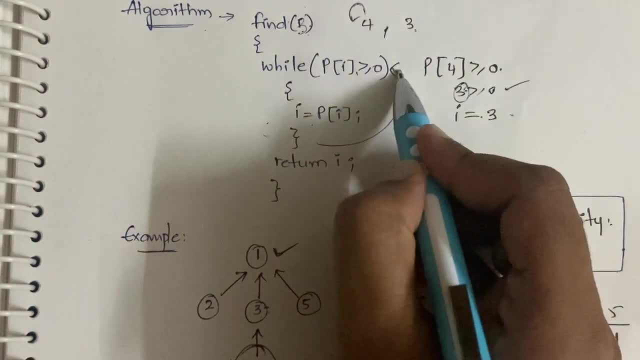 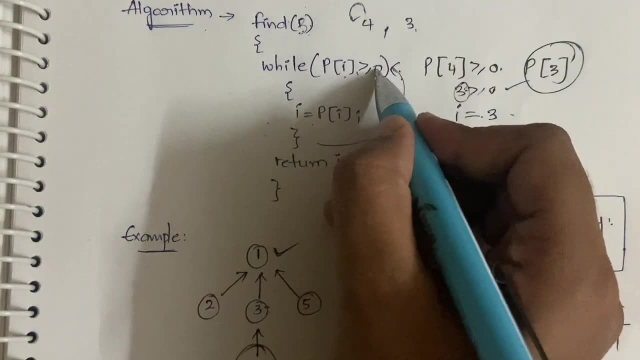 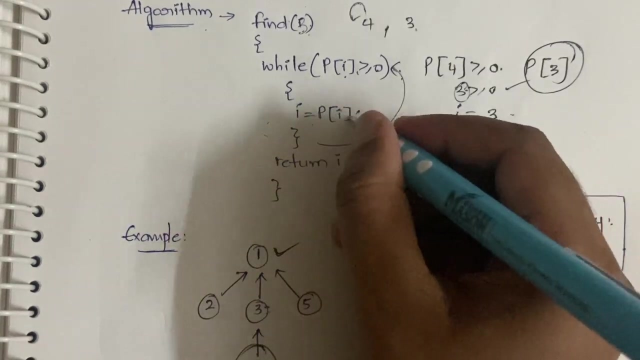 parameter is three, while p of i is greater than or equal to zero. here, what is p of i in this iteration three? what is parent of three? one, one is greater than or equal to zero, true, so this? you will come to this statement, so i will become one now. i, because i is equal to p of i. p of i is equal to how much one, so i is equal to one. 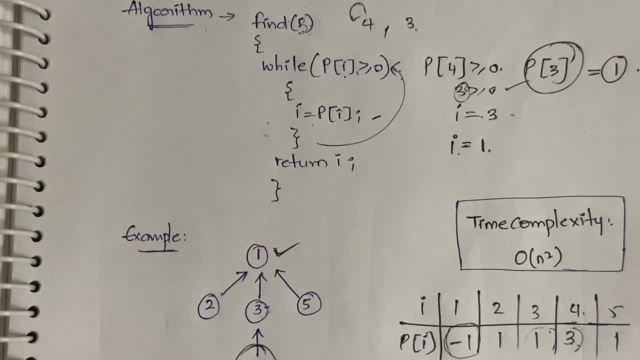 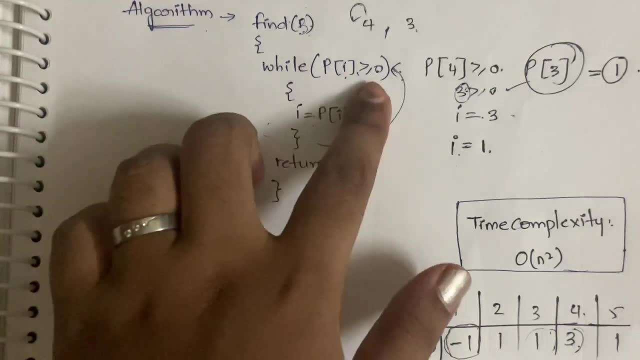 you are again passing one here, so you are trying to find one. okay, while p of one is greater than or equal to zero, what is p of one minus one minus one is greater than or equal to zero. no, this is false, so you will come out of this while loop. 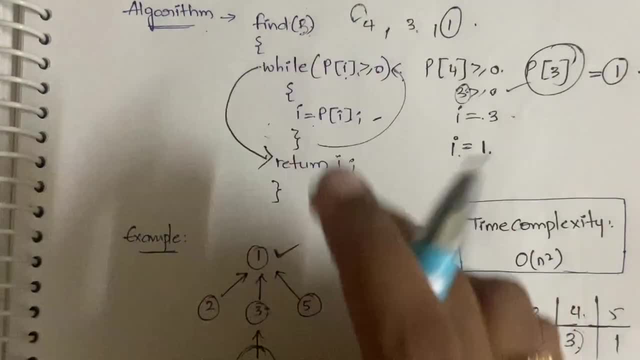 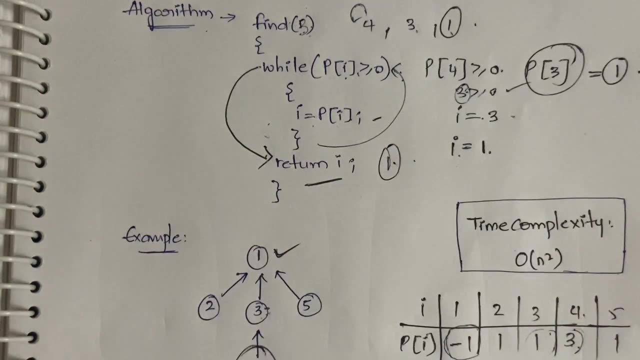 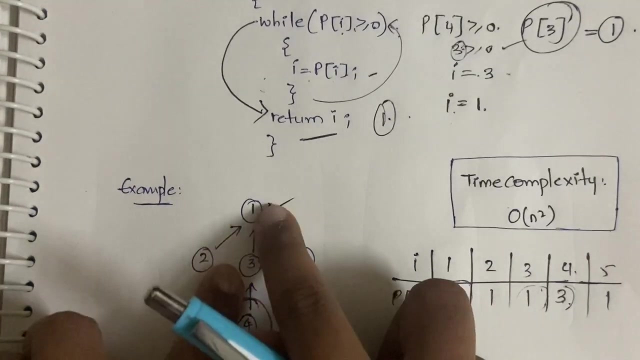 okay, so one is our present, i value right, and then it will return: i what is our present, i value one. so it is returning. one simple. first, you will find the parent of four. parent of four is three, yes, it is greater than zero. so you will go for parent of one. parent of parent of three. yeah, parent of one. 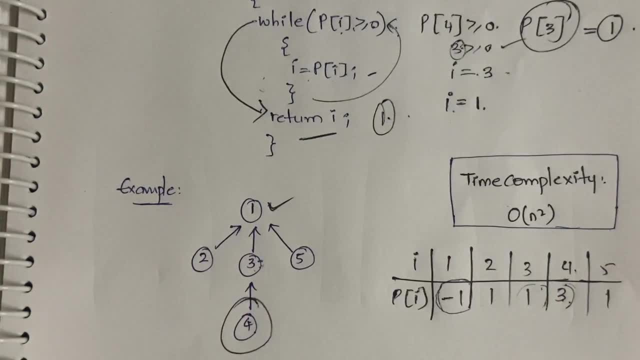 is minus one. minus one is not greater than zero, so obviously you will return one. okay, this is about find algorithm. so that's all for this video, guys. let's meet up soon the next coming video with another topic. thanks for watching the video till the end. if you're still having any doubts, let me know in. 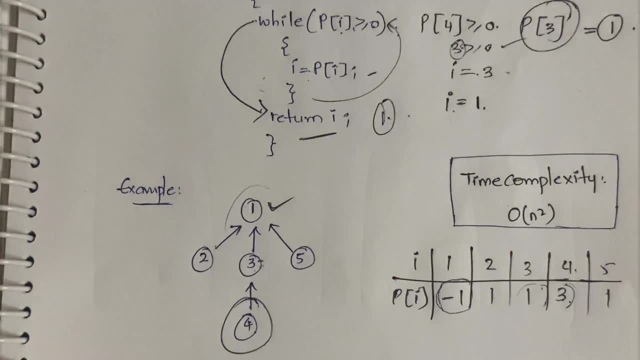 the comment section. let's meet up soon in the next coming video with another topic. 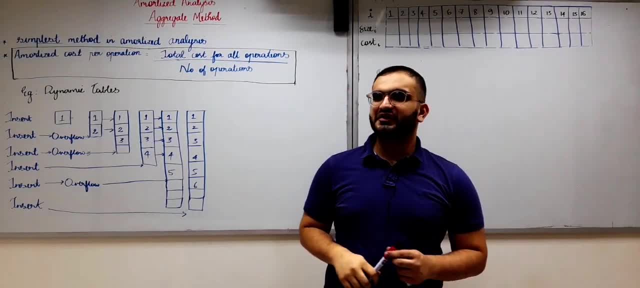 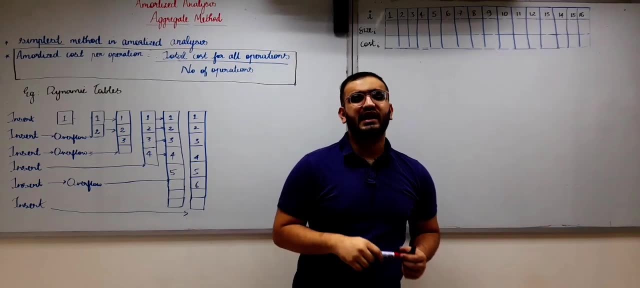 Hi friends, welcome to my channel. So in this video we are going to see the first method of amortized analysis, that is, the aggregate method. If you have not seen the previous video, I recommend you to watch the previous video where I have introduced amortized analysis From this. 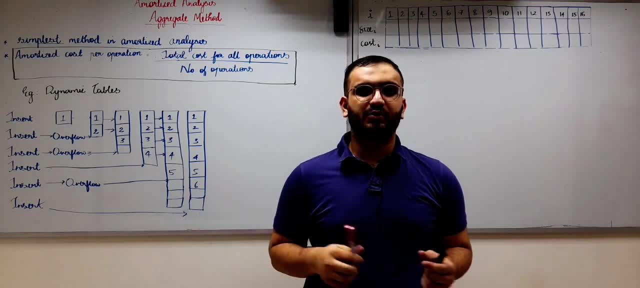 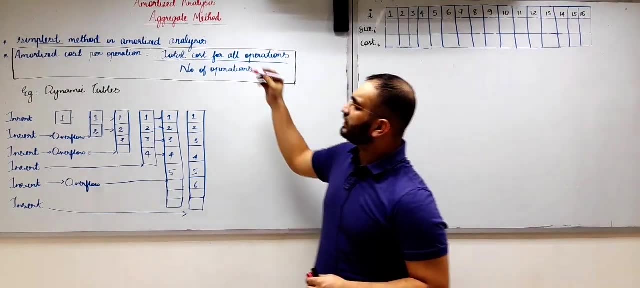 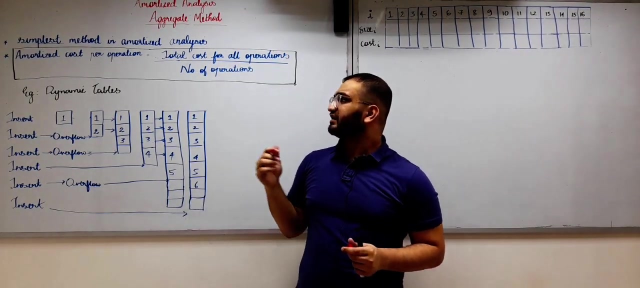 video onwards, I'm going to talk about the different types of amortized analysis, And right now, let's talk about the first method, that is, the aggregate method. Now, as it is written over here, aggregate method is basically the most simplest method of amortized analysis And the